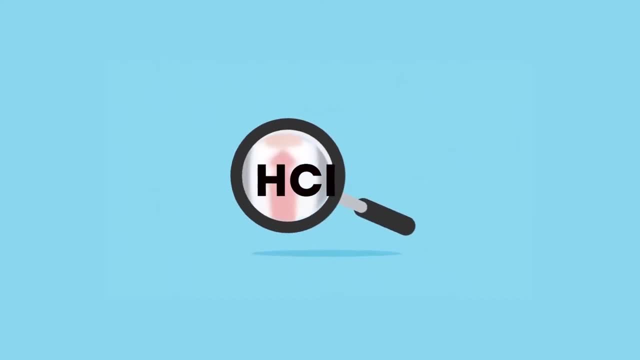 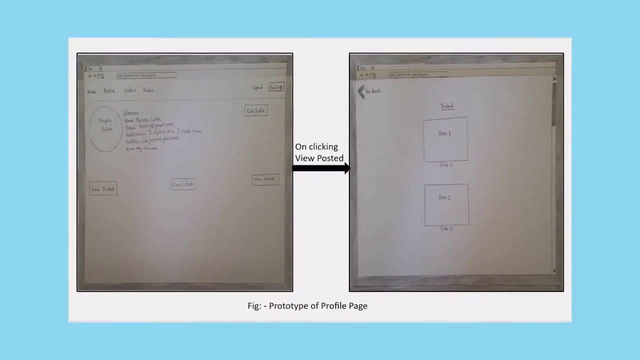 make our solution even more effective. we approach the system design with HCI design principles. The rest of these two weeks involve study and documentation of our case. Starting with Week 3, we entered our design and implementation phase. Initially, we developed our first paper prototype that encapsulated the concept and drew the designs. 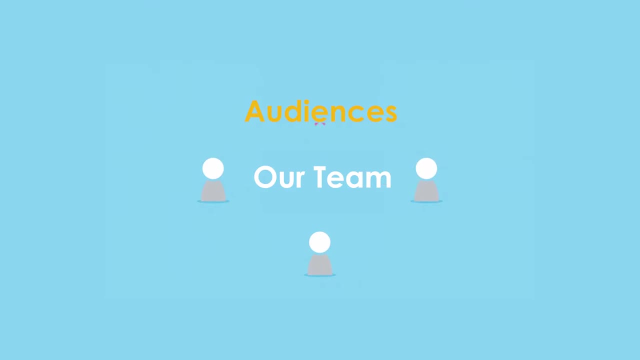 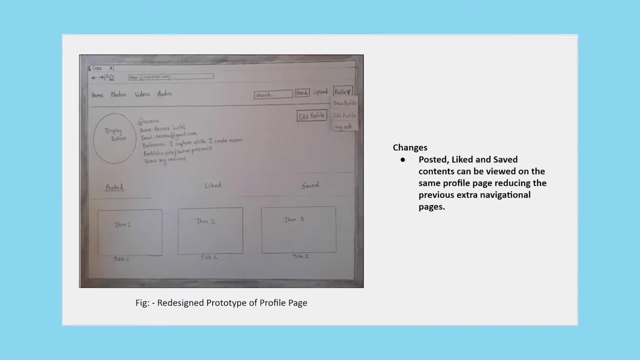 that best supported our concept. In the first week we developed a three-page paper prototype, was then introduced to our targeted audiences. their feedback and suggestions were recorded. we incorporated those feedbacks and redesigned our final paper prototype. in week four, we designed our initial ua design based on our final paper prototype, which was then subjected to heuristic. 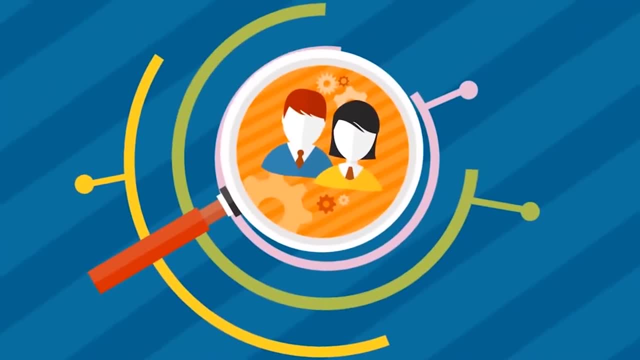 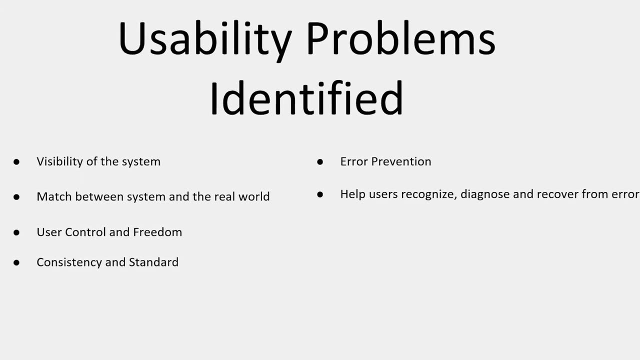 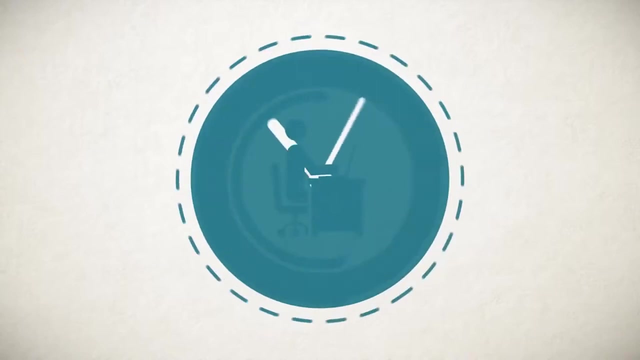 evaluation, our usability inspection method, where another group named tabler evaluated our interface and identified different usability problems that a user is likely to encounter, based on jacob nelson's principle of interaction design. starting week 5, we conducted personas, fictional characters, based upon our research, to represent different types of users that might use our platform, which 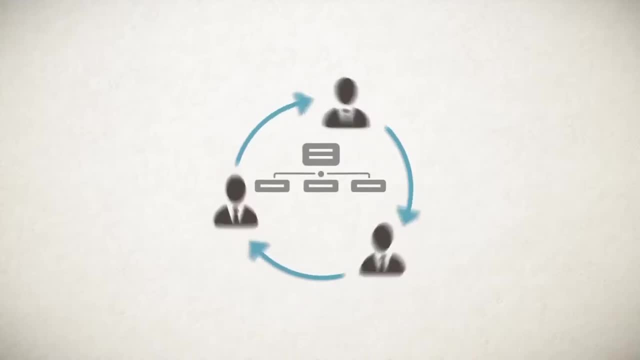 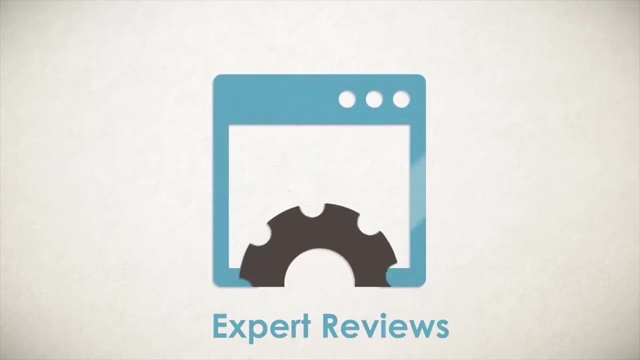 help us understand our user needs, experiences, behavior and goals. the final ui design was developed using schneiderman's golden rules and norman's design principles, where earlier usability problems were tackled and new ui design aspects were incorporated to develop an efficient and usable website. expert reviews through consistent inspection were conducted at 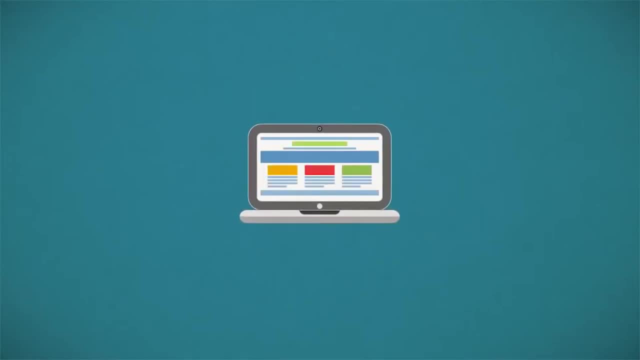 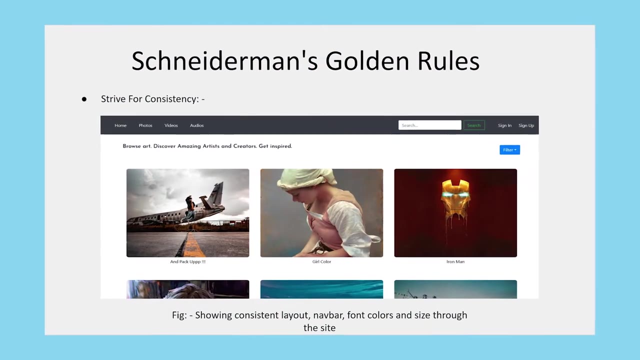 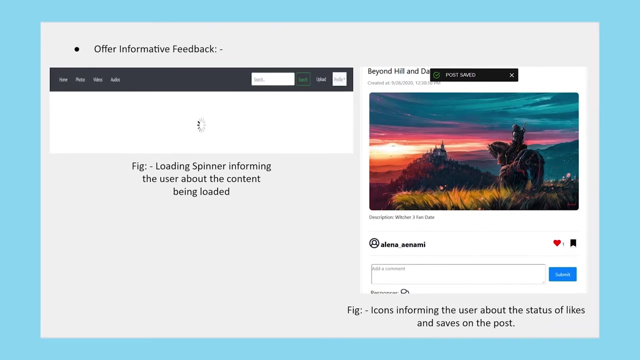 documented. a fully functional website was now developed as a minimum viable product. let's see how this design will incorporate it. to maintain consistency, our system has similar screen layout, typefaces, fonts, colors and many hierarchies. to offer informative feedback, we have used navigational feedback animation and alert to inform user about the action performed. 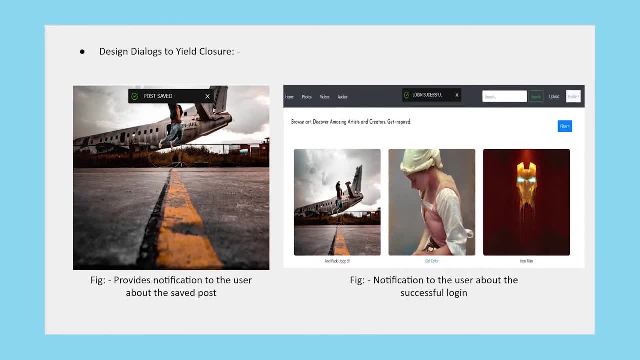 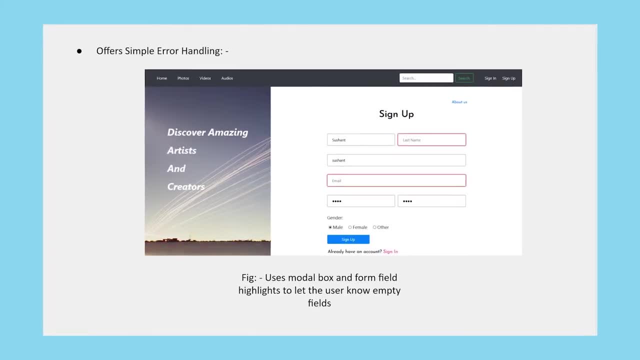 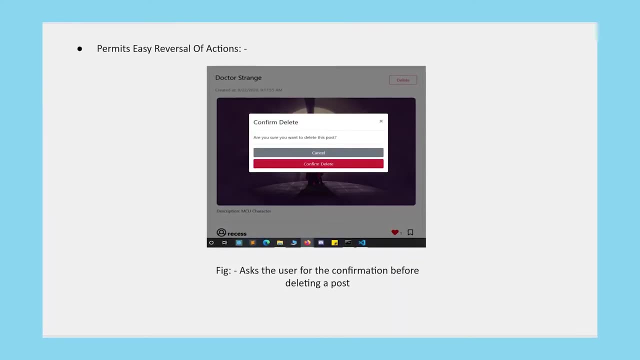 for design dialogues to yield closer. our system indicates the start process and end of the action through pop-up menus, loading spinner and push notifications for simple error handling. we integrated from validation techniques and alert messages permits easy reversal of accent. for easy reversibility of action, our system asks for confirmation so that the user may not delete. 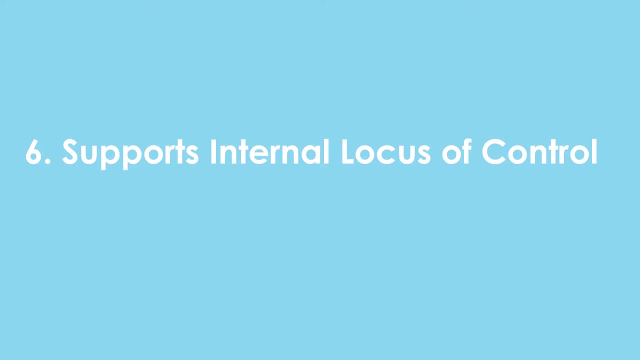 something accidentally. to support internal low cost of control, our system leaves it upon the user preferences to include portfolio link and profile pictures to reduce certain memory load. our system has consistent layout with proper information hierarchy maintained. similarly, we have used ton norman's six principle of design to address the identified problems, which consists of: